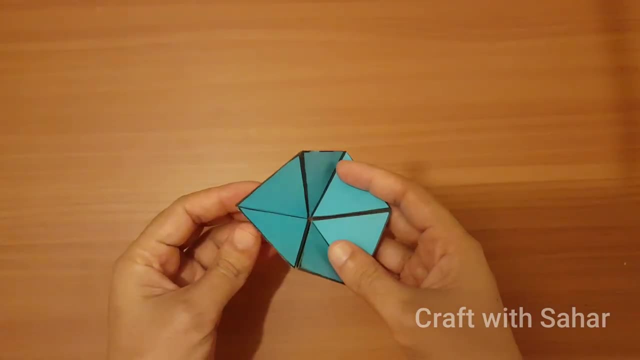 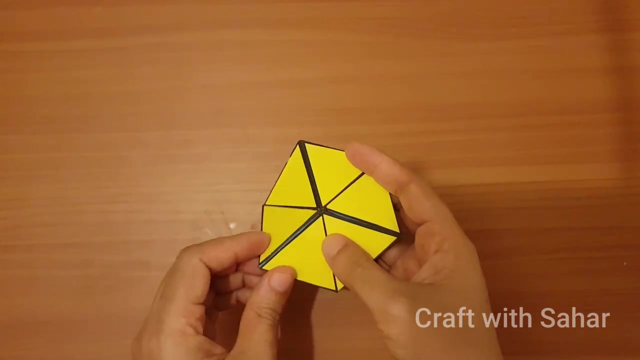 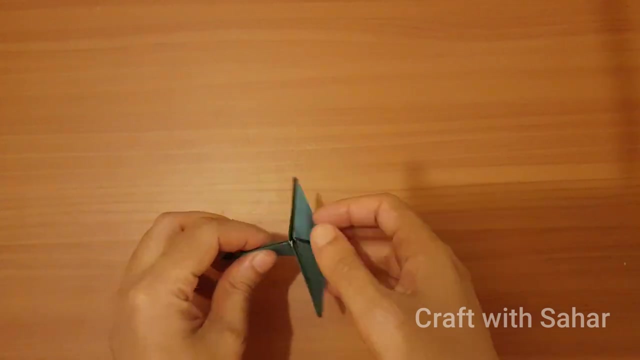 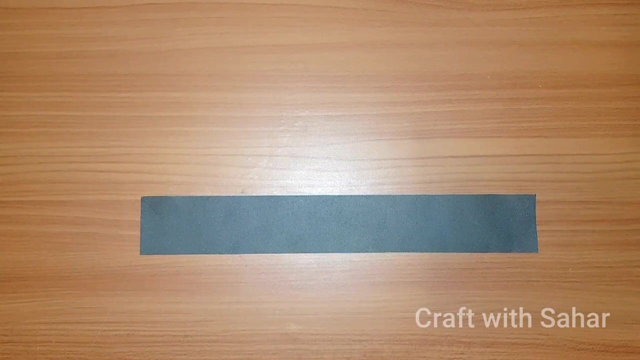 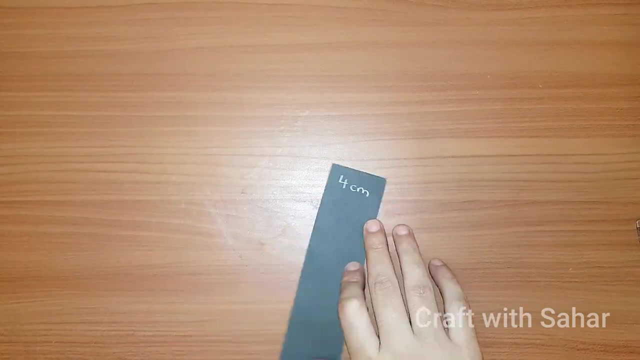 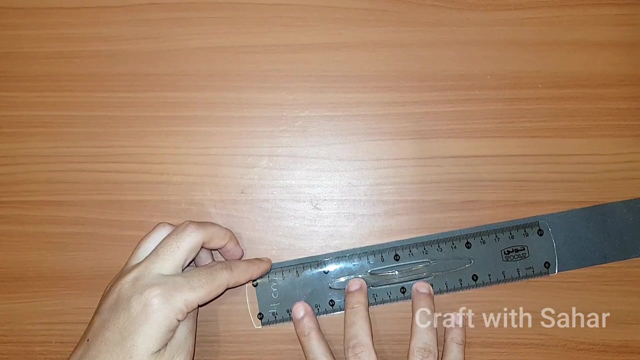 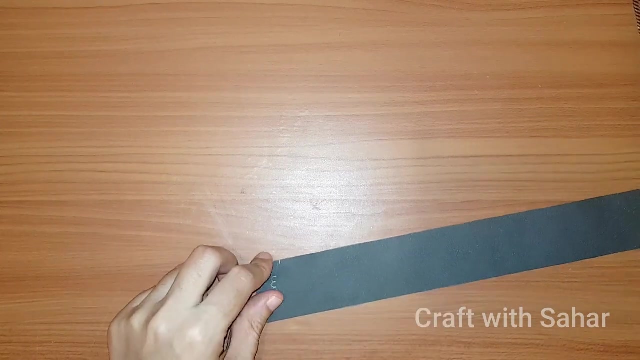 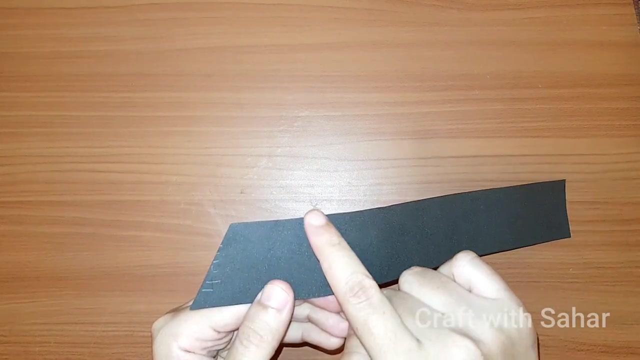 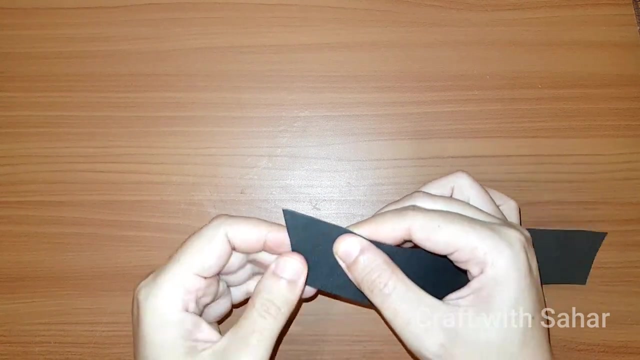 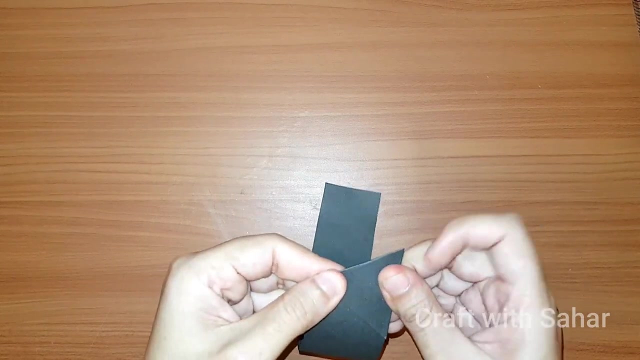 Please re-enters the screen. You can now edit the editable audio file As a proper video. you can edit the audio files to an MFA format. Here you can adjust the quality of your video. Thank you, Thank you.